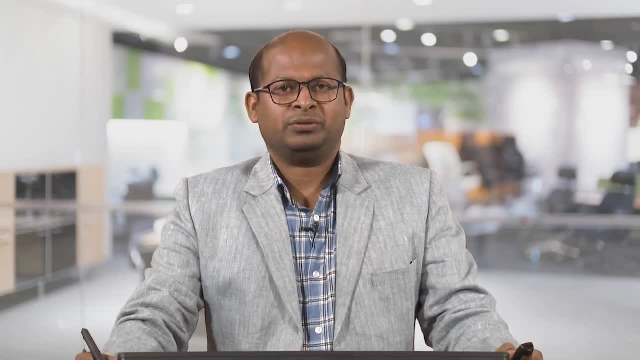 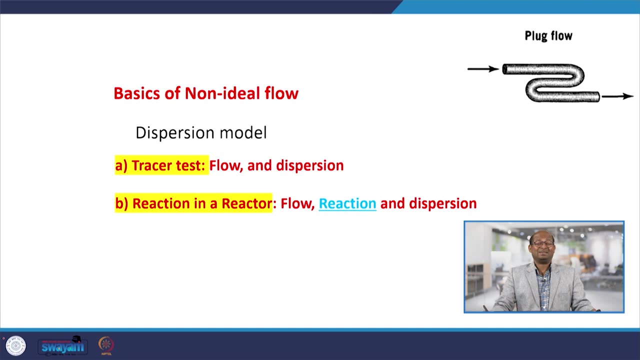 use for a reactor that we are going to design or we are designing. So whether the reactor is ideal or non-ideal, or up to what extent it is non-ideal, So that we can discuss, Check. or whether the reactor is close to ideal or not, So that we can check. So for 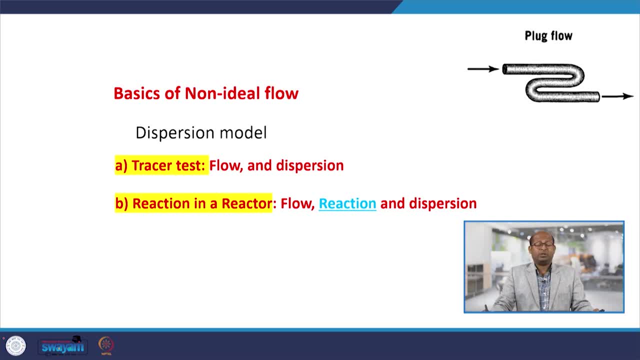 that various models means that we already have discussed, So there are so many models. that is, the segregations models, tank in series models that we have discussed in your previous class. So today we will discuss about the dispersion models. So in the dispersion. 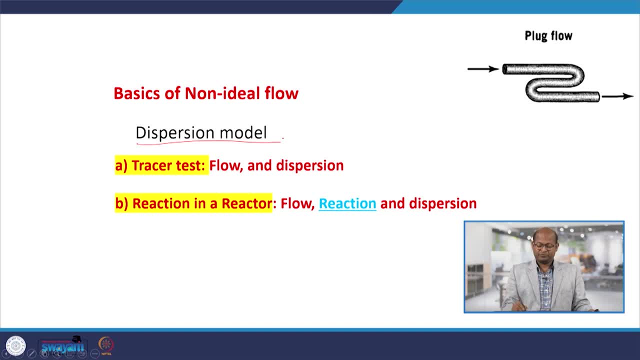 models. let us say we have a plug for reactors, or any reactors, When reactant molecule may pass from here, that is entering here and that is after reactions. it is leaving as a product from exit of the reactors. So this is the reactors here. this. 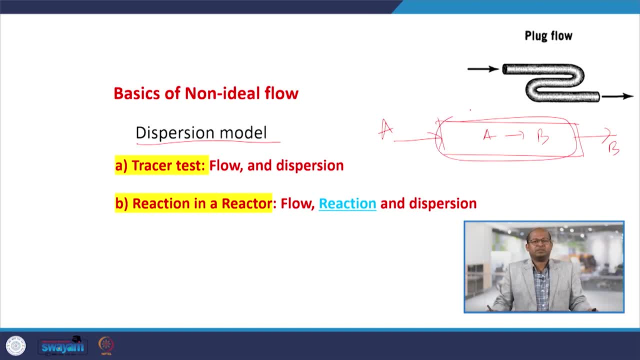 is a reactor that we have designs for a particular or specific reactions. So now we are going to discuss about the tracer test. we have discussed- So that is the tracer test- what is the requirement of the tracer test. So that is the tracer test. what is the requirement of the tracer? 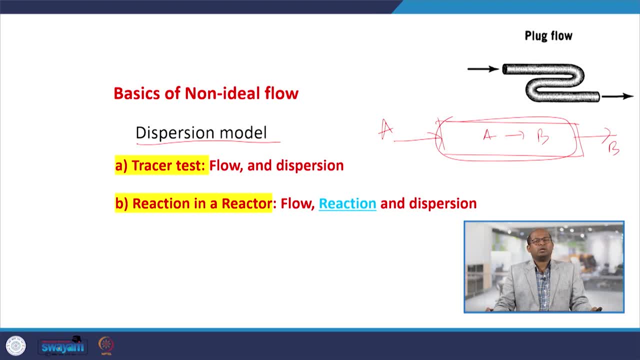 test. That tracer test will tell us about the RTD of that particular reactor, or residence time distributions of the molecules when it is flowing through the reactors. So are the non-ideal nature of the reactor that we can get from that. So various way you can measure. So here dispersion model we have chosen and today 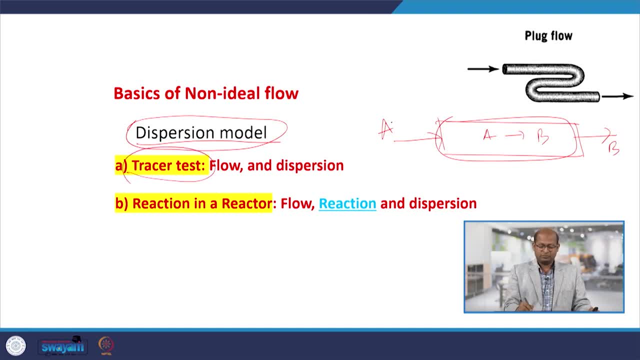 we will discuss dispersion models. So let us say we have a tracer test, So instead of A, So if we pass any tracer, that is, we can say T, Let us say concentration, So we can say concentration of tracer, that is Ct, So that we can inject here instead of A. 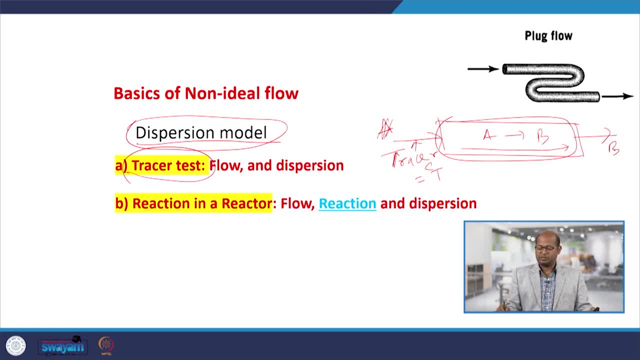 So then the tracer can pass through this reactors and from the exit of the reactors. So tracers we can collect at different interval of times. So that way we can measure whether the tracers, at what times that is coming or leaving from that reactors. if we plots and 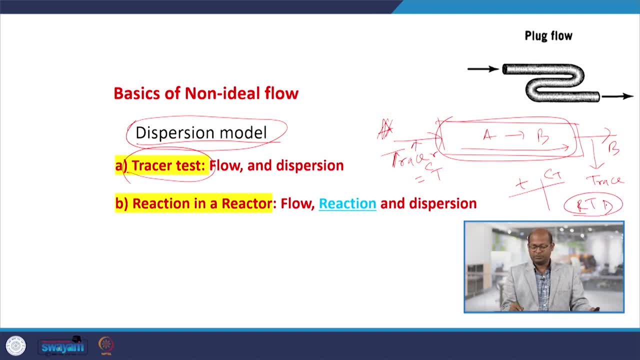 from there we will get RTD or residence time distribution function. So when normal flow is there inside of the reactors, so molecules moving from one direction- left hand side- to the right hand side, So it is normal flow is there. So this is the plug: flow or normal. 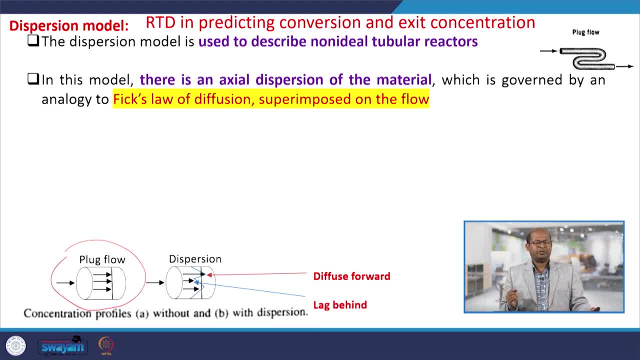 flow when molecules moving from one point to the another point. So with that, when molecule is moving, let us say tracer is passing from here and it is leaving tracer here. So tracer molecules following this pathway it is leaving from there. So it is the normal flow or convective. 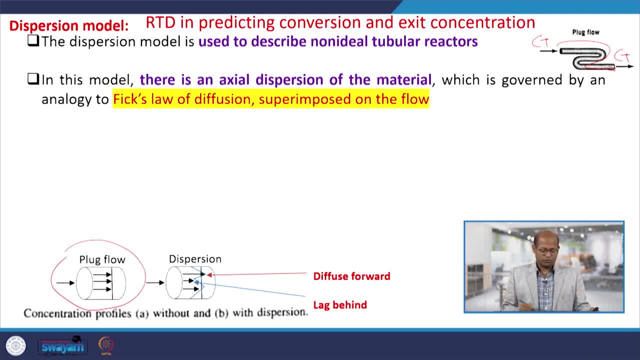 flow that we can say So with that. so molecular diffusion is also there, so with that. molecular diffusion means when molecule is moving from inside of the reactor from one point to the another point so there is a possibility of dispersion. means few molecules diffuse forward and few molecules 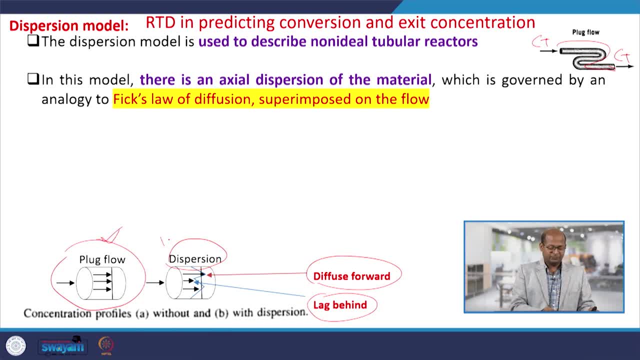 lag behind. that is called diffusion. This is the basic difference from here. this is the normal flow. there is no diffusion. and if diffusion does exist inside of the reactors, when molecules moving from one point to the another point, so as a result, what would happen? so if diffusion does not exist, so then all. 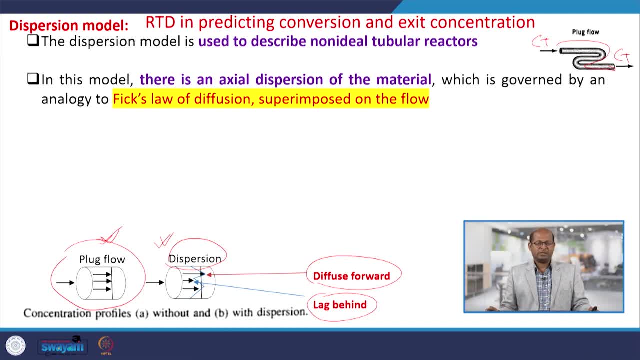 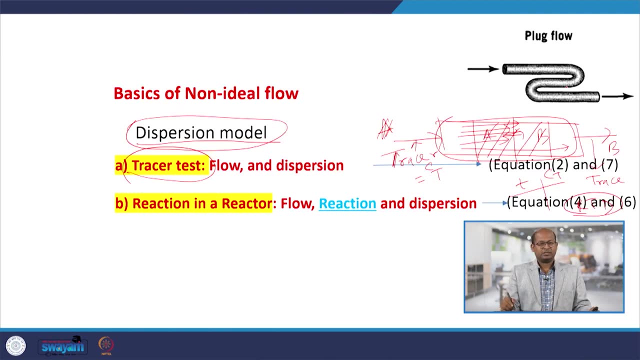 molecules spent equal time inside of the reactors for the reactions. So if diffusion exists, so few molecules spent longer period of time. few molecules spent smaller time inside of the reactor. So therefore offerals means whenever we conduct any reaction. So in this reaction, 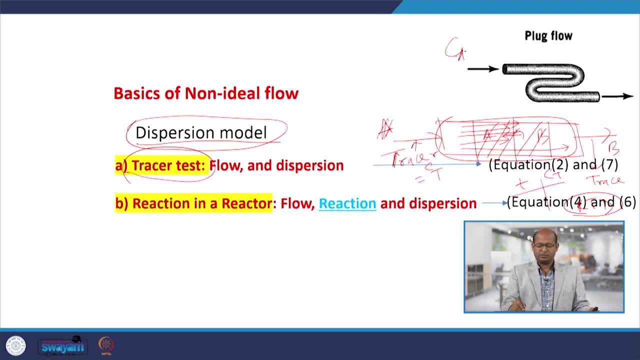 So after, if we conduct any reaction. so then, so what we measure, Ca naught, that is the inlet concentration, Ca is the outlet concentrations and based on that we can measure thus conversions for this particular reaction. So if this Ca is very important means when it is moving inside of the reactors, so if 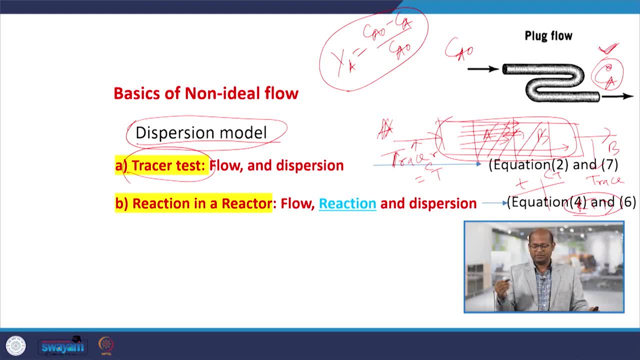 diffusion is there, then this concentrations would vary. So actual concentrations will not get due to the diffusions. So once we do not get actual concentrations, then conversions would be different, So actual. So that is the main things for the non-ideal nature of a reactor. 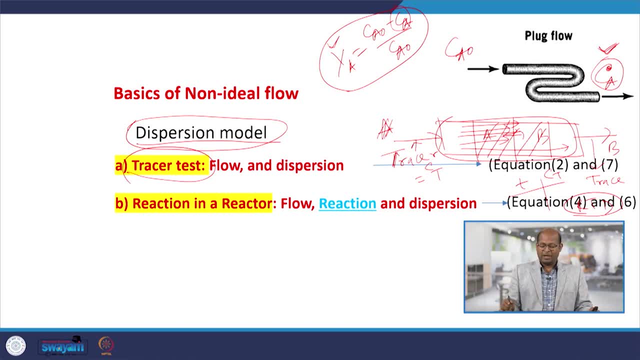 So due to the diffusions, are diffusions affected? So at the beginnings, two way we discuss this. dispersion models. first one is the tracer test. In the tracer test, when tracer is there inside or passing through the reactor, there is no reaction. So only tracers will pass or flow from one point to the another point. 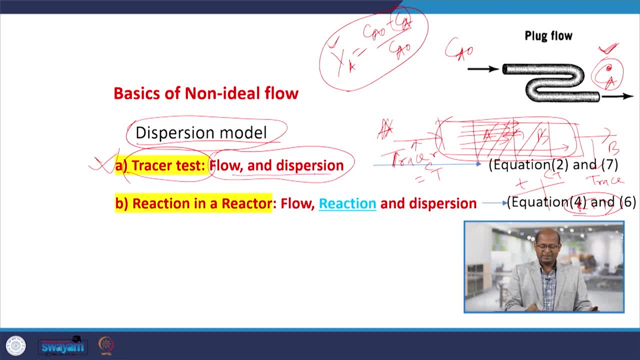 So only tracers will pass or flow from one point to the another point, And with that there is no reaction. So that is the main thing. With that dispersion should be there, And when same reactors we are using for a specific reactions, So when we conduct these reactions here also, molecules will flow and dispersion also will. 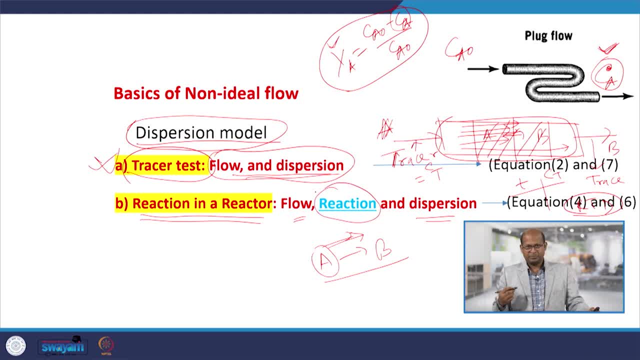 there At the same times, additional parameters or the observations, that is, the reactions. So in flow and dispersion, this is for tracer, and when reaction is there with flow and dispersion, reactions should be there. So therefore these are the key things. So for this tracer test, we will evaluate few equations and when reactions is there, for 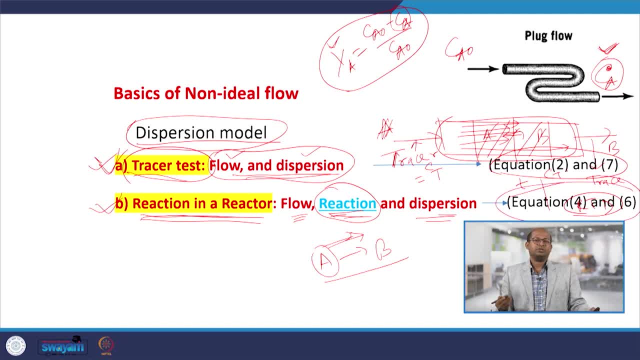 that also, we derived some equations And those equations we will derived after that, using some boundary conditions. we solve that equations to find out what would be the if dispersions exist or diffusion is there. considering these models, what would be the concentrations of the reactants or if and? 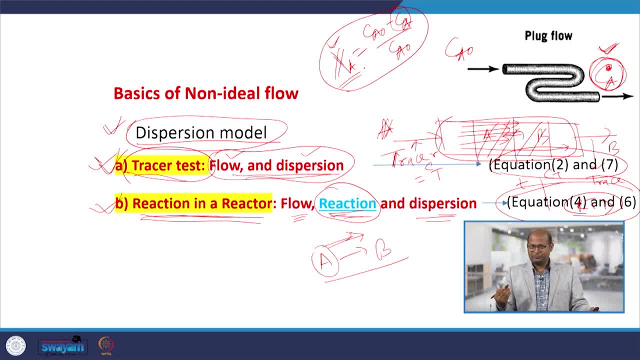 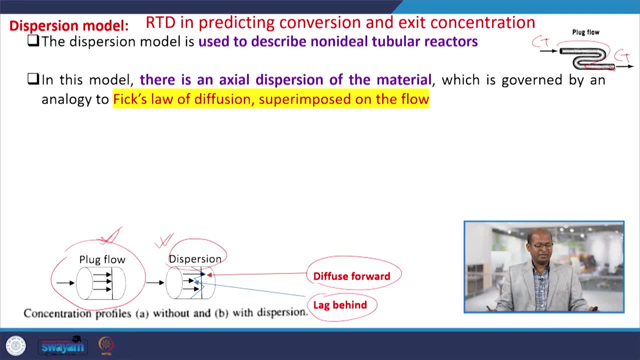 based on that, conversions that we can predict. So this is the key thing, So that one by one, we will discuss how the model equations we will direct, considering that dispersion models. So when dispersion is there, means molecules is diffusing from one point to the another. 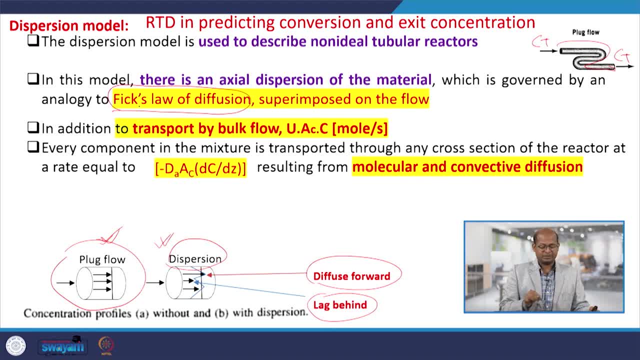 point. So for that fixed law of diffusion we have to consider that fixed law of diffusion, that is molecular diffusion from one point to the another point inside of the reactors or any confined space. So that would be superimposed with the flow. normal flow is there with that diffusion. 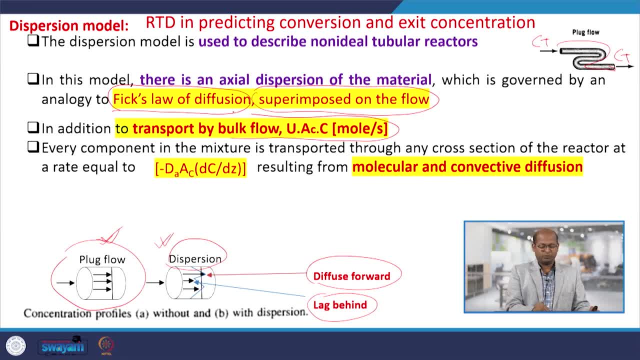 So normal flow or bulk flow when molecules is moving from one point to the another point. so this bulk flow or transport, by bulk flow we can express U, AC into C: C is the concentration, AC is the cross sectional area and U is the superficial velocity. that is the way means. 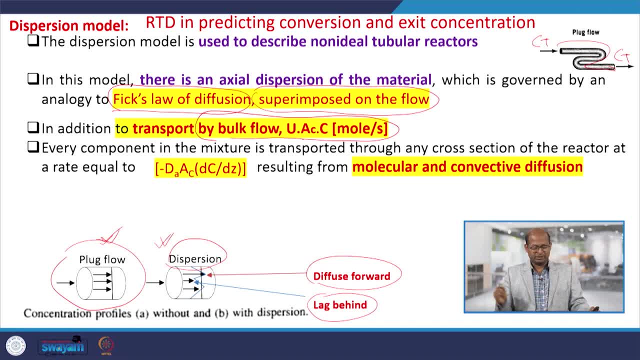 molecules moving from the velocity moving from one point to the another. Hence that molecular or convective diffusions that we are using or expressing from the fixed law of diffusion is this minus DA, AC, DC by DZ. So here C. maybe if we use treasure C we can write DCT. if C equals CA, if C would be CA when. 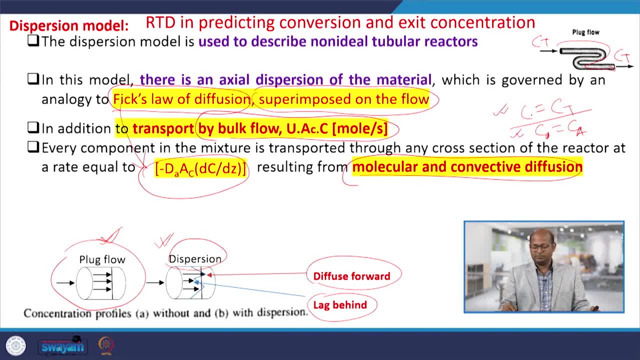 reactions means these are the things, both the way we can express the concentration. when only treasures will be used, C equals to CT. we will consider when reactions would be there. CA: we will. C- we will consider as a CA. this is the thing. So now these are the two things we have. means bulk flow and so molecular or convective diffusions. 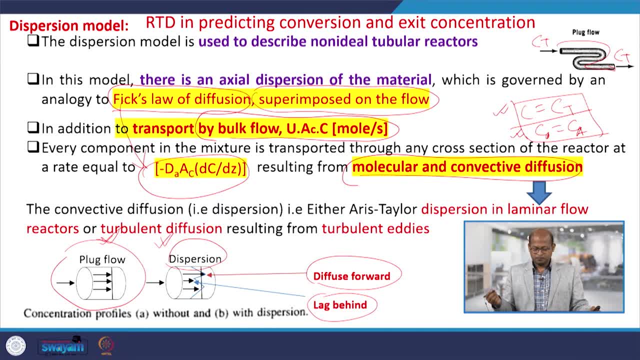 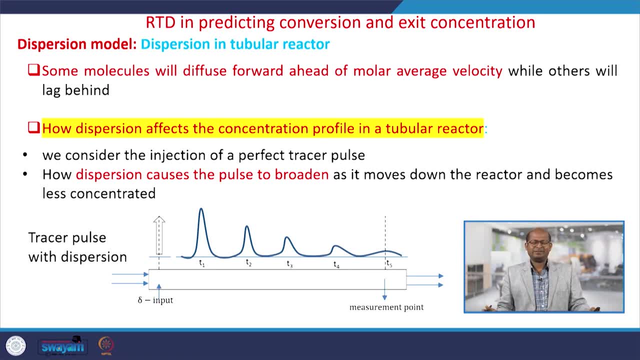 the things we have. So now means when molecular diffusion is there, when flow is there. So then response of treasures. suppose we are injecting a pulse treasure in the inlet point of that particular reactor flow lines. So then the response would be like this: So this is the response: curves, but when dispersion is there. so what it usually happens with times. 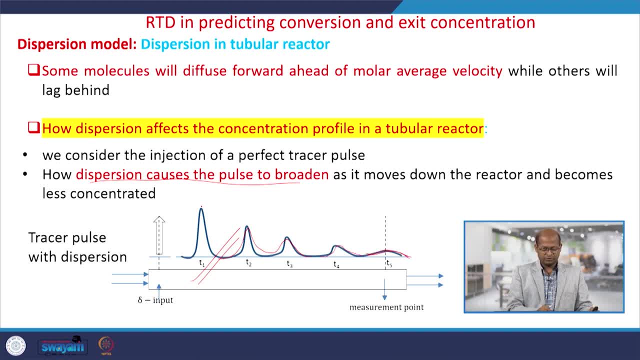 it is broaden. So this is the broaden. So here peak and here peak, Here there is peak, sharp peak is there, but here it is broaden. So these responses, or the molecule is moving from one point to the another point, So there is the means due to the dispersions, this peak broadening is there. 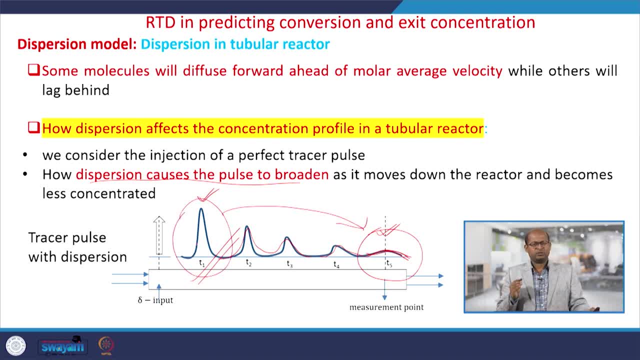 So this is actual. So if there is means no diffusion exists, So then the responses will get a perfect peak, but it gradually decreases and it is broadening. So that is due to the dispersion. Diffusion or dispersion exists in when molecules is moving. 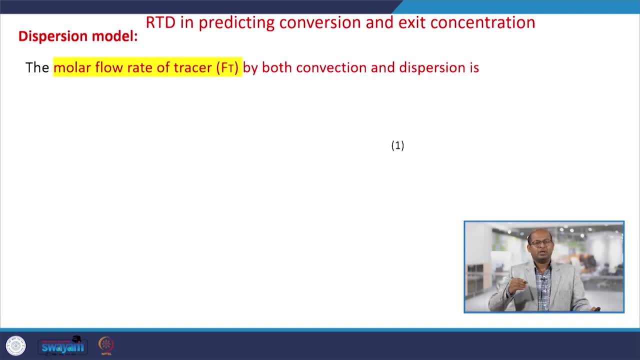 So then this type of things happens, or the nature of responses curves would be like this. So now, molar flow rate of the treasures means first we will consider, discuss by considering treasures and then we will consider reactant. So there are two components, Ct and Ca. 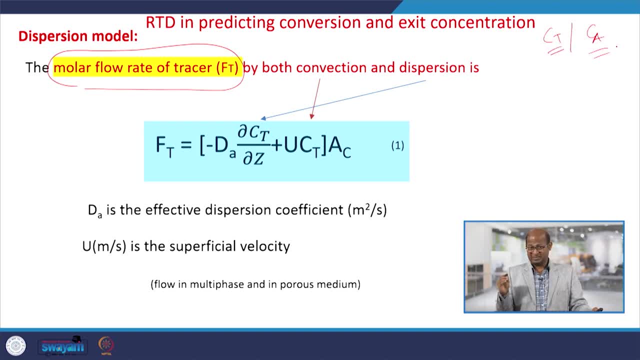 Ct is the treasure and Ca is the molecule. So Ct is the molecule, Ca is the concentration of reactant. So first we will discuss whatever, that is, the treasures. So molar flow rate of the treasure, that is, we are expressing in terms of Ft. 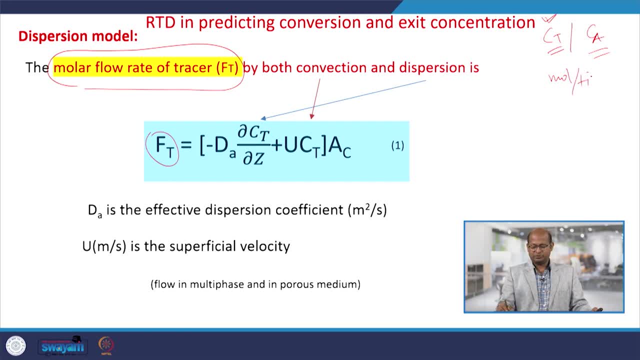 Ft is the mole per unit time, So the treasures that is flowing from one point to the another. point that we can write Ft: Ft equals to right hand side, that is, this part is the diffusion means and this part is convective flow. So u Ct, Ft. 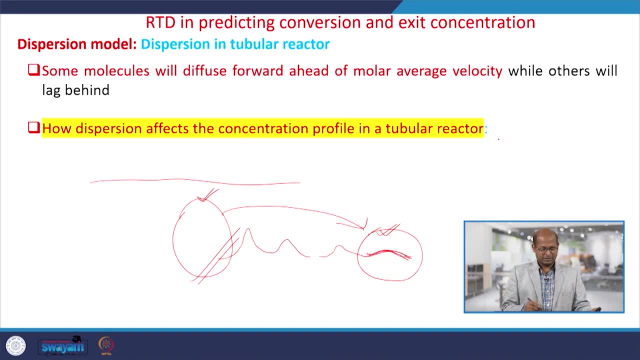 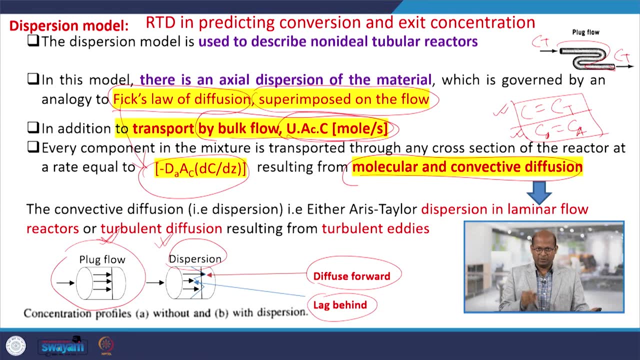 So u Ct, So u Ct, So u a C that we have discussed. this is u a C. that is the means for bulk flow, the molecules or molar flow rates of molecules, mole per unit times, that molecules moving from one point to this, and this is due to the diffusion- both will combine. 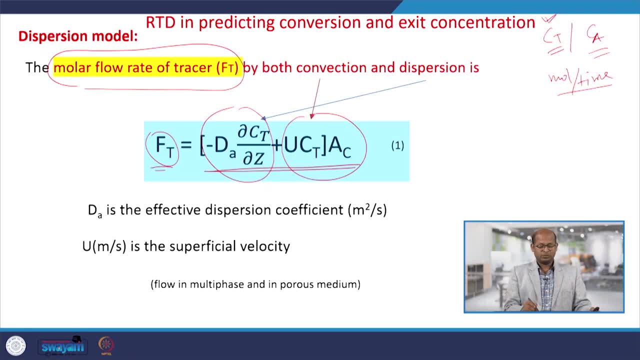 So then diffusion plus molecular moments, both will be there. So molar flow rate of that treasures due to the convection and dispersion that would be combined. So equation one is the combined. So here dA is the effective dispersion coefficients, it has units and U is the superficial velocity. 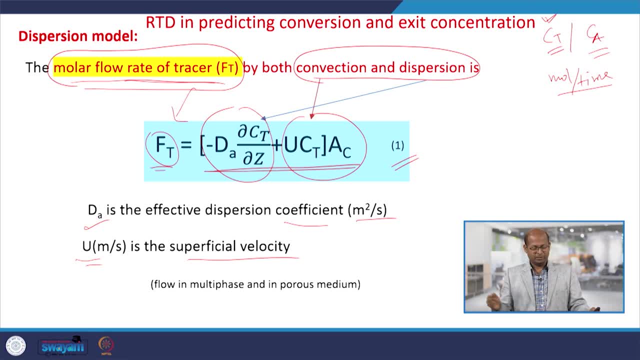 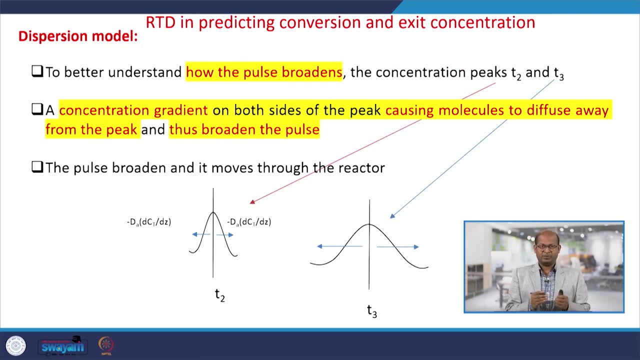 that way means molecules is moving from one point to the another point, So superficial velocity we can express this way. So now broadenings of peaks. that is due to the how the pulse broadens, So a concentration gradients at that particular, both the sides of the peak, causing molecules to diffuse high. 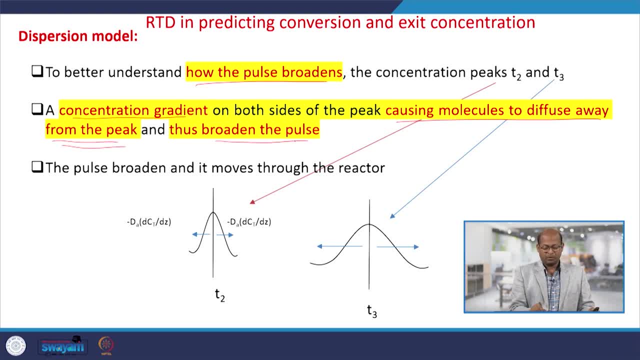 from the peaks and therefore the peaks would be broadens, or pulse would be broadens. So pulse, why it is broadens? So, from this particular point, this is the centre. from here to it is from both the sides. the molecules diffuse from the centre. So therefore it is broadens. 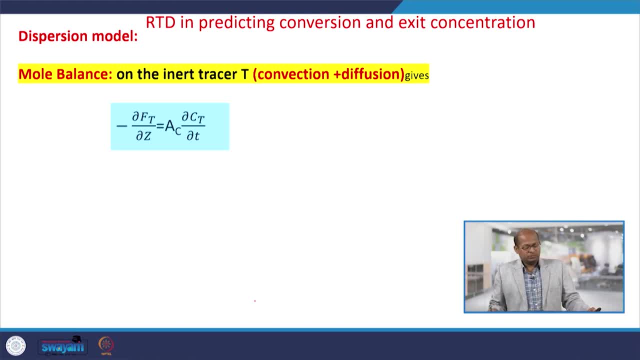 So this nature of the peak should be like this. So now mole valence means the tracers molecules. it is moving from one point to the another points. So convexions is there and diffusions is there. So we are going to do the mole. 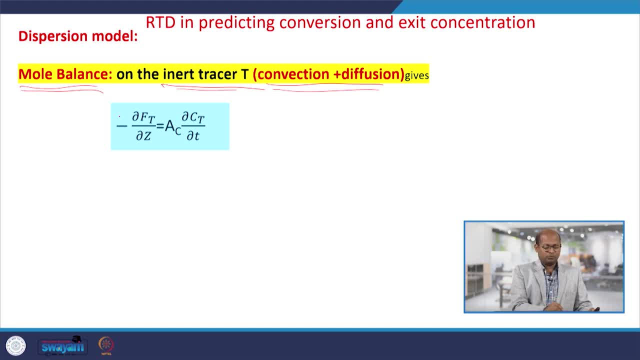 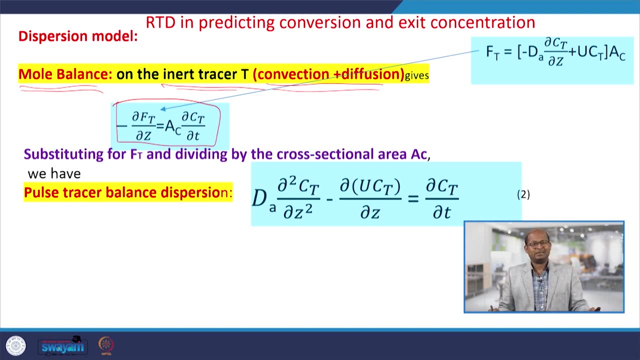 valence balance on the inner treasures components. So mole balance equations is this: So minus del Ft by del Z equals to Ac del Ct by Dt. This is the mole balance equations. unsteady state mole balance equation for treasures when it is moving from one point to the another. 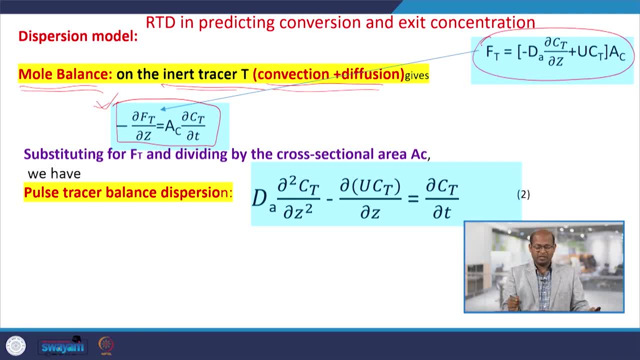 points And this molar flow rate components, this we have just discussed. So this is due to the diffusion and this is convective flow or bulk flow. So this Ft, if we substitutes here this Ft, molar flow rate, so this is due to the diffusion plus bulk flow. So this 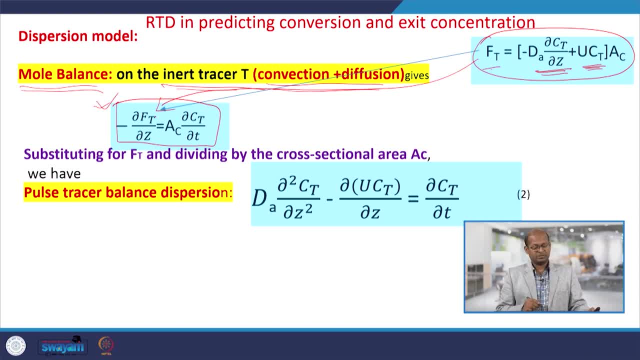 Ft, if we substitute here in the mole balance equations, so then after substitutions and if we dividing both side, left hand side, right hand, with the Ac, and then after simplifications, a second order, differential equations. So that is the Ct is the concentration of the treasures I said, and dA, that is the diffusion. 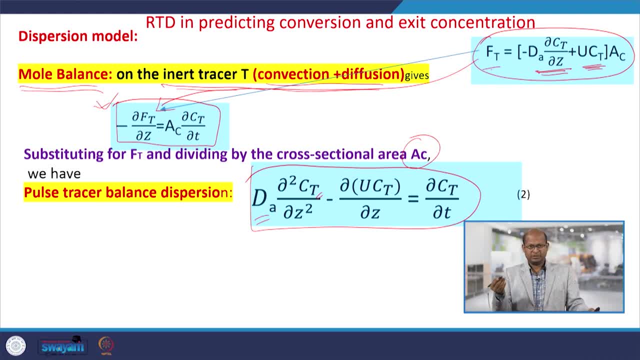 or coefficient. So that is dA, we know means in the mass transfer. we usually study that. So equation to pulse, treasure, balance, due to the dispersions, these equations we have to use, So one equations for treasures and mole balance from the mole balance equations. 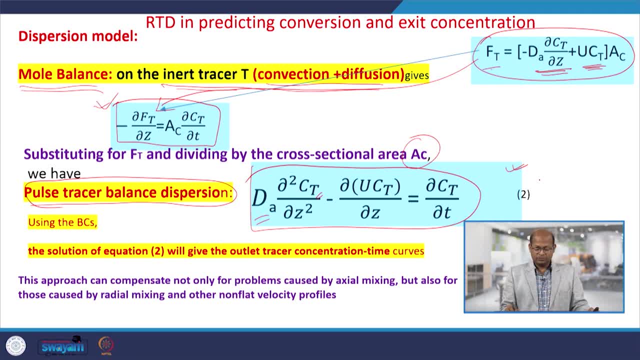 we obtain this. So these equations if you want to solve, so we need some boundary conditions. So this is the second order differential equation for the pulse treasures, when there is a dispersion, so with the bulk flow. So these equations we have to solve using some. 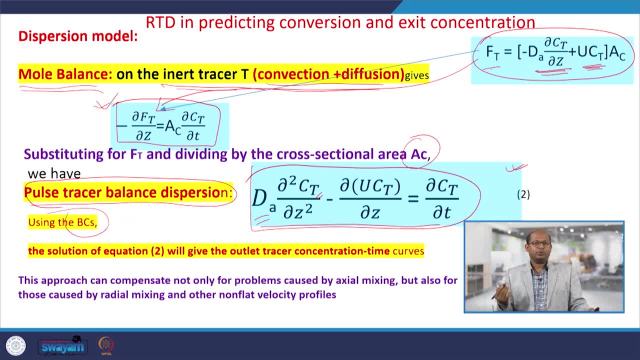 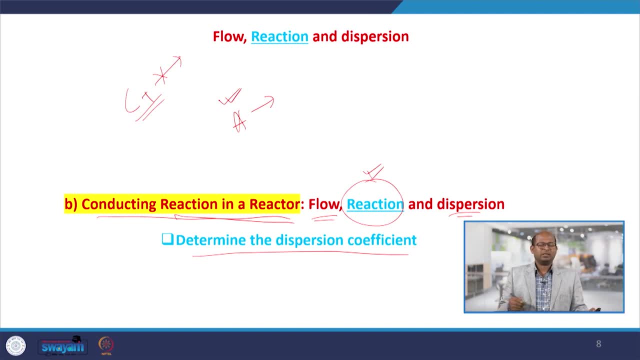 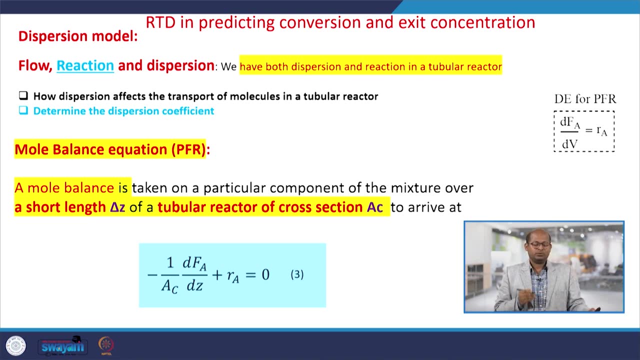 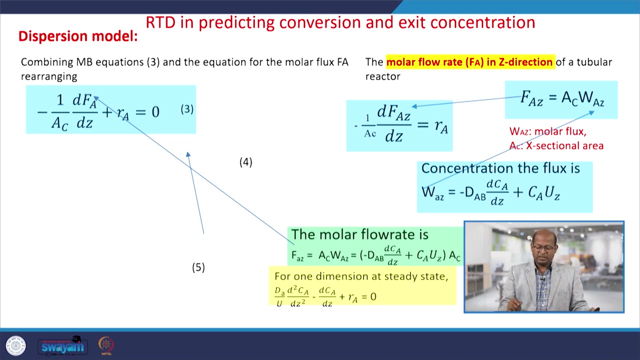 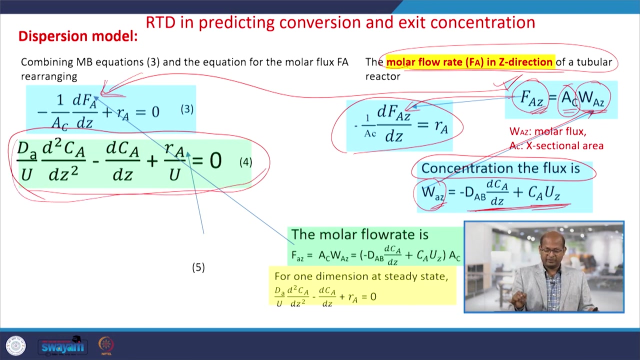 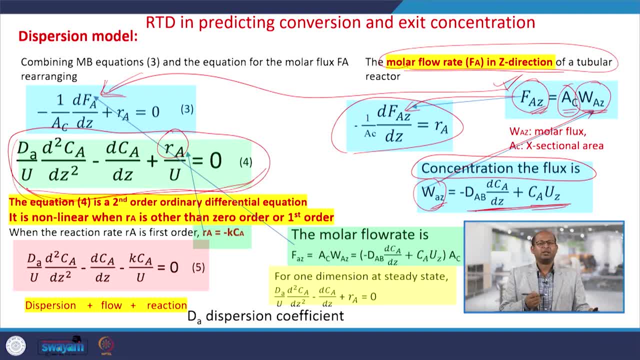 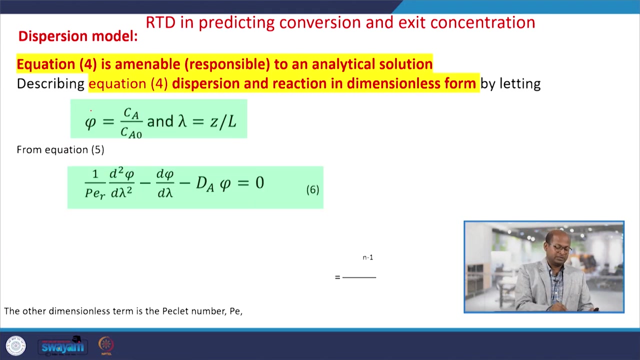 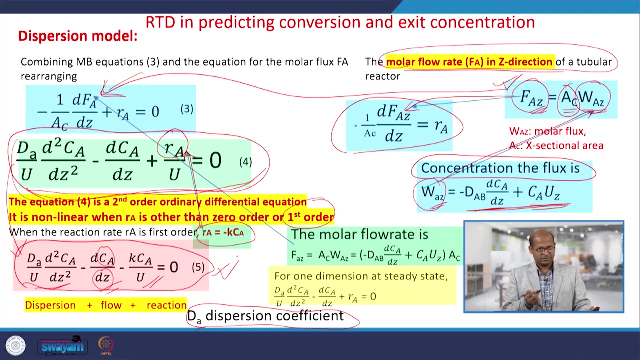 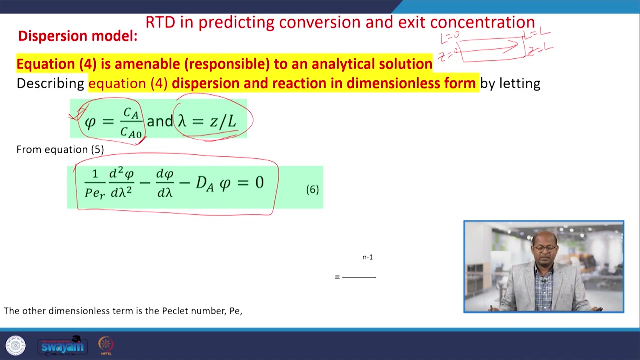 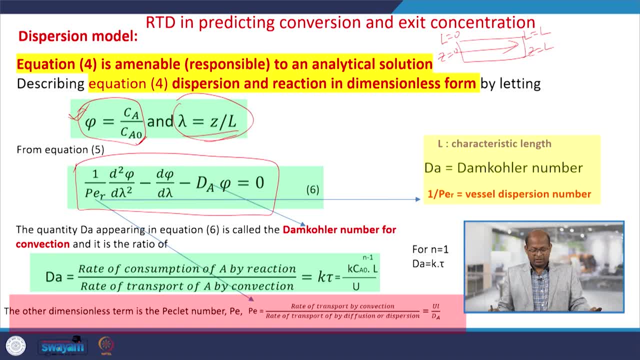 form equations we have derived. So here is small da. that is the Damkohle number that also we have studied. Damkohle number for first order reactions we can express: da equals to tau into k. So tau is the space times, k is the reactions rate constant. So for first 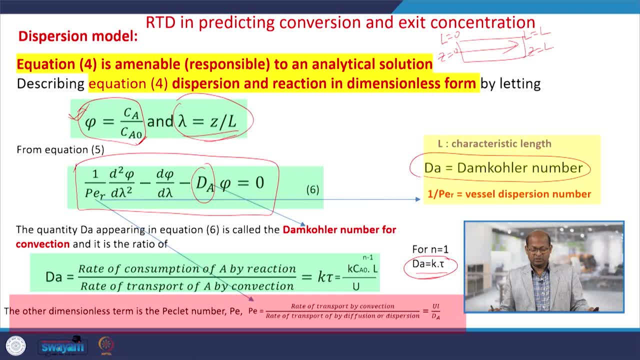 order reactions. da equals to k into tau, that is the Damkohle number. and here another component or parameters or number is there that is called Peclet number. So the Peclet numbers we can express in terms of ul by da. This is the Peclet number. So 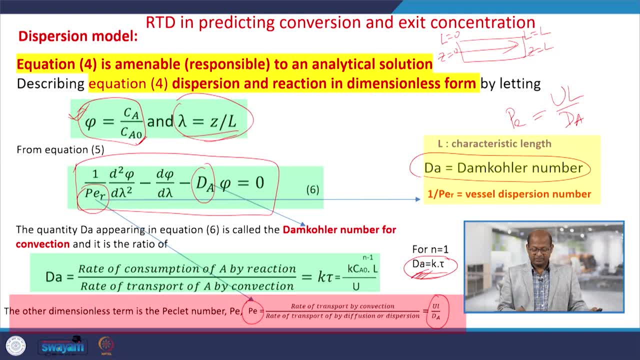 here this da and this da is different. Here this da is the Damkohle numbers d, small a. Here da capital A, that is diffusion coefficient. Both are different, So you should mention this da coming from the diffusivity terms. Diffusivity or diffusion, or the terms which 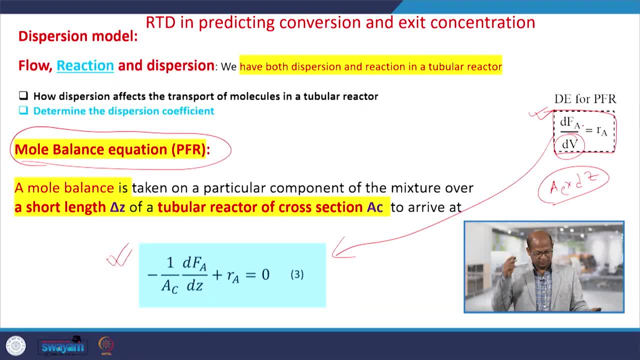 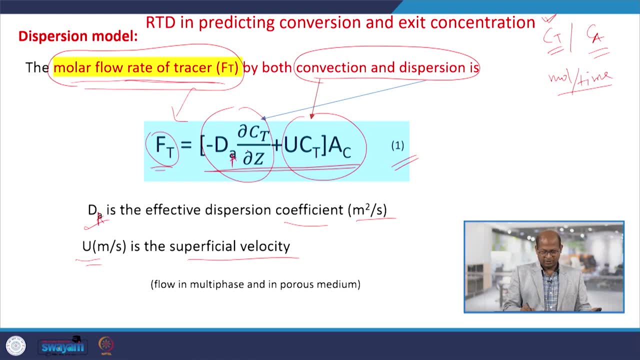 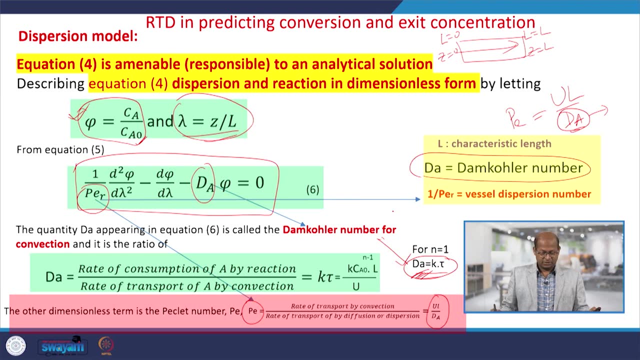 comes. So I discuss diffusion parameters. So that is this. dispersion coefficient, effective dispersion, This is da capital d actually, so meter square per second. Now we have dispersion, Peclet number and dispersions Here. this will be Damkohle number. This will be small a. 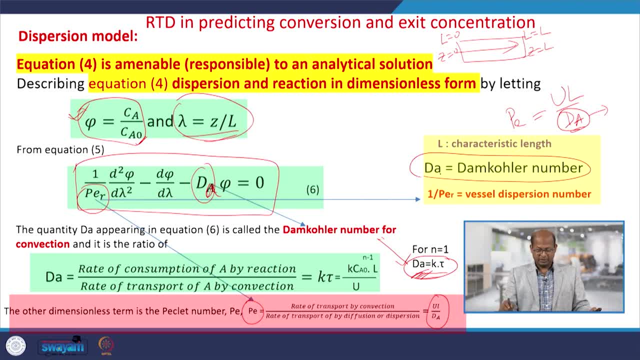 Damkohle number 1, this Damkohle number and Peclet number. So now we know this dA rate of consumptions. it signifies the Damkohle number signifies rate of consumptions of A by reactions upon rate of transport of A by convection. So that is the k? tau. we can express this way for first. 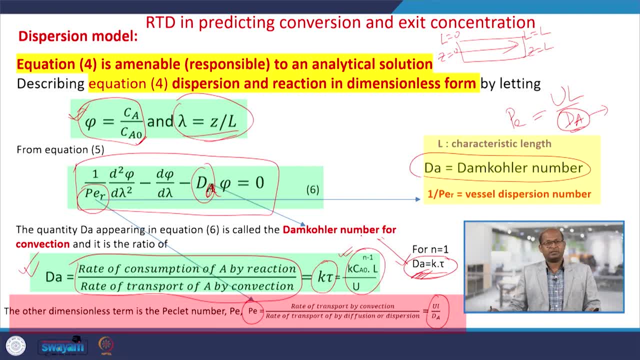 order reactions. So this is due to the consumptions of reactants, A by reactions and this is transport of A, it velocity or superficial velocity indicating. So we can express or elaborate this one. So then we can say that dispersion or Damkohle numbers, that is, rate of consumptions of A. 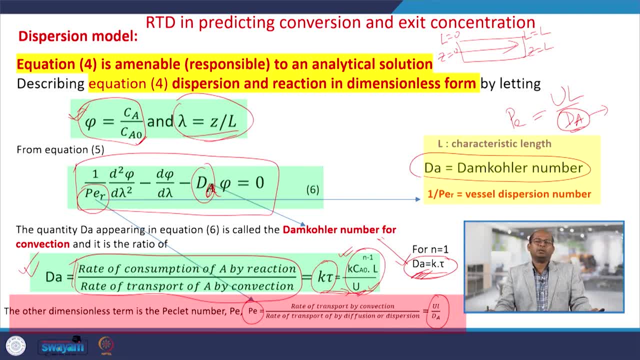 by reactions, to the rate of transport of A by convection. So that signifies or indicates and Peclet number. so what is rate of transport of A by convection to the rate of transport by diffusion or dispersion? so ul by dA, So that indicate Peclet numbers. 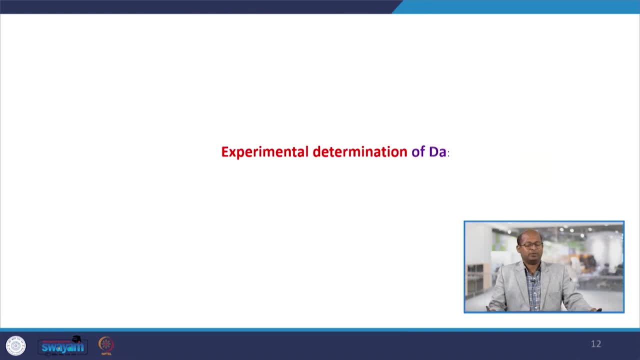 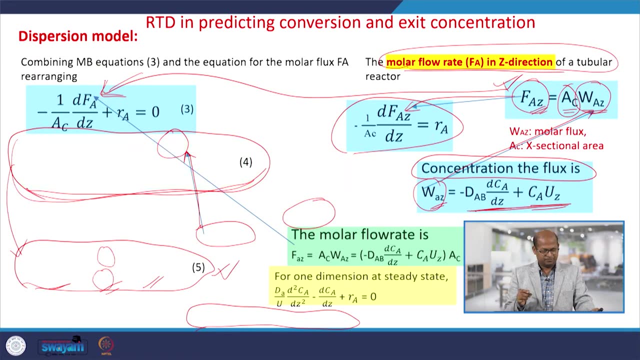 So these are the Peclet numbers and means Damkohle numbers. how that is signifies So now means two equations we have derived. equation 6 we have derived for reactions and equation 2 has derived, but we have not converted this into dimensionless forms. later we will convert. 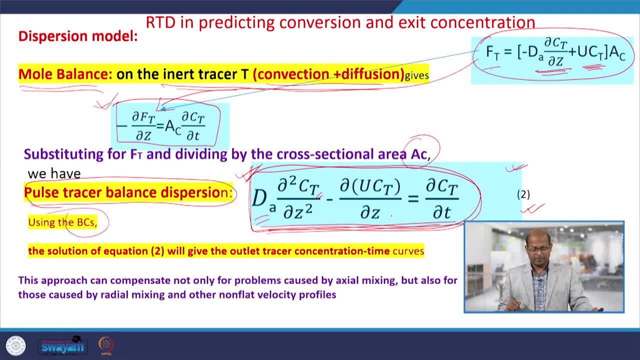 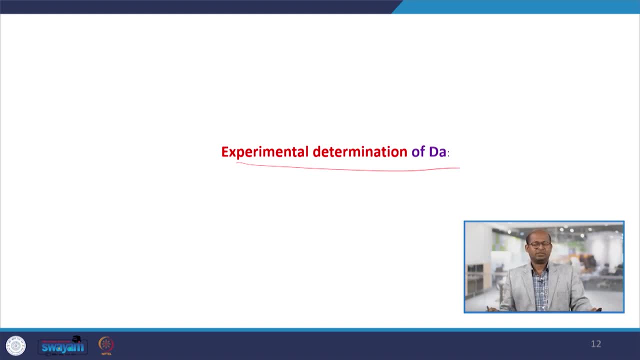 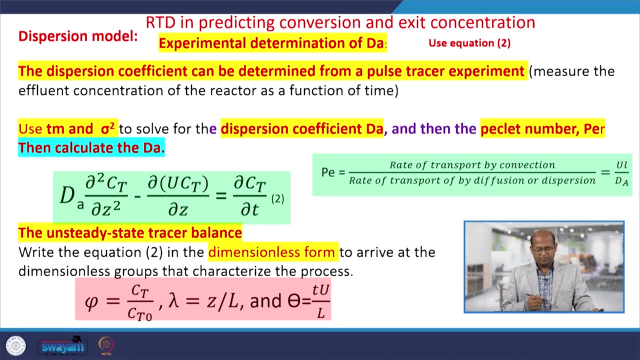 into dimensionless forms also. this is for treasures. So now experimentally, how can measures dA, dA is that dispersion numbers or dispersion coefficient, experimentally? So then we can find out. Ok, So we have means when we have studied at the beginning. so this: 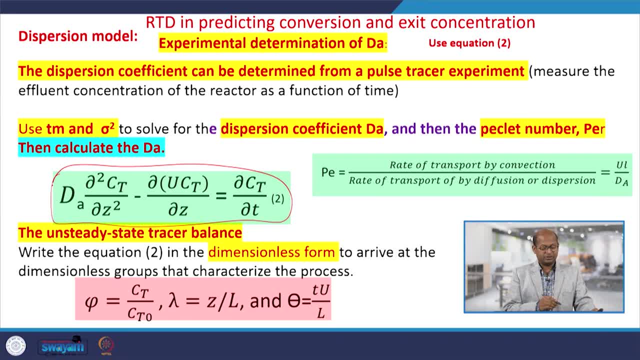 is from the treasures, the equation 2 that we derived, so that equations also we have to convert into dimensionless forms. ok, So then treasure concentrations and dimensionless distance we can write. and then if we convert these equations in, by converting dimensionless parameters, So, and theta equals to dimensionless. 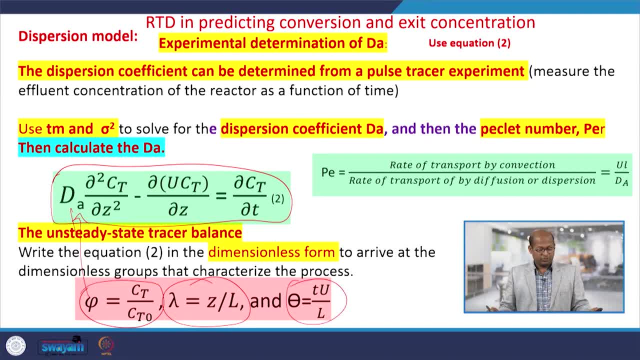 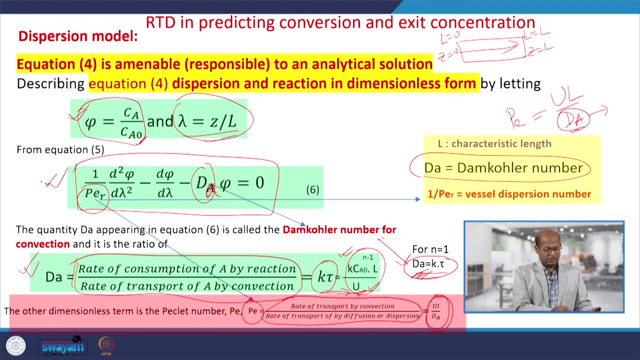 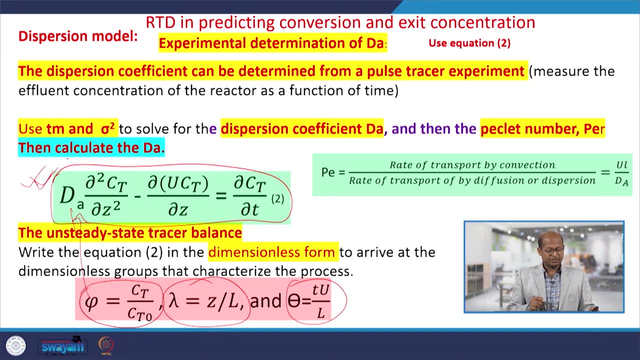 time ut by L. So here is equation 2 from tracer test. it is coming, and equation 6 that is coming from reactions. So now means when these equations we are converting into dimensionless forms by considering dimensionless concentration and dimensionless distance for the tracer test. So then it would become this: 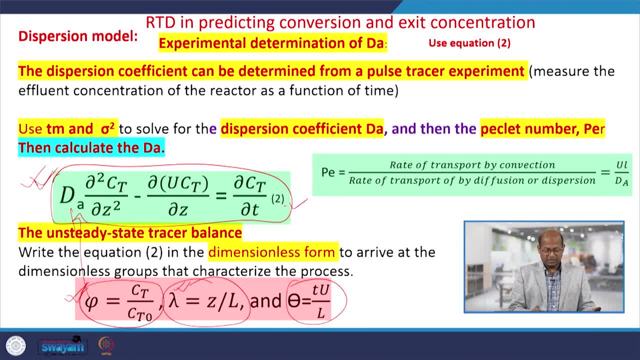 equation 7.. So these equations 2 we are converting into dimensionless forms by using psi and lambda. psi is the dimensionless concentration, Ct by Ct0,. Ct0 is the initial concentration of the tracer that we are injecting when pulse injections is there and Ct is the tracer concentration. 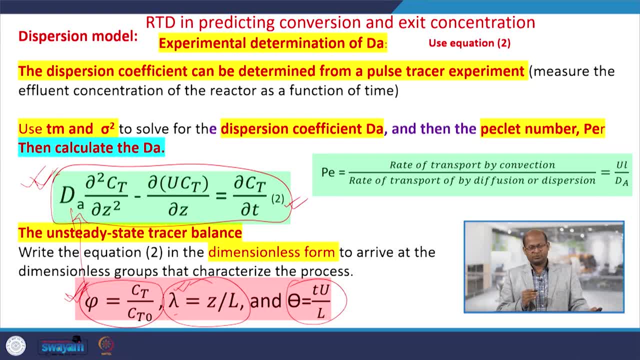 at different time, So along the length of the reactors, when it is moving the tracers, the concentration at different location of the tracer would be different. So therefore, the psi, or dimensionless concentration of the tracers, we can express this dimensionless parameters, or length, we can express. lambda equals to this and this is dimensionless time. 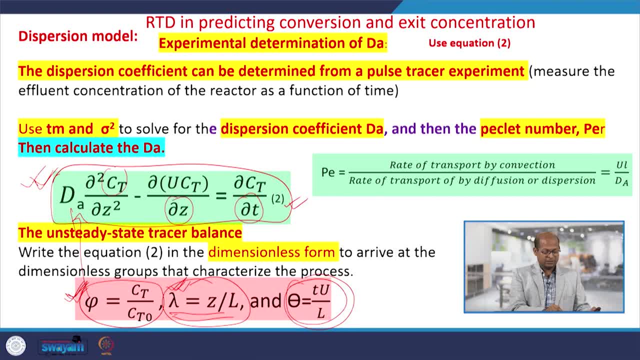 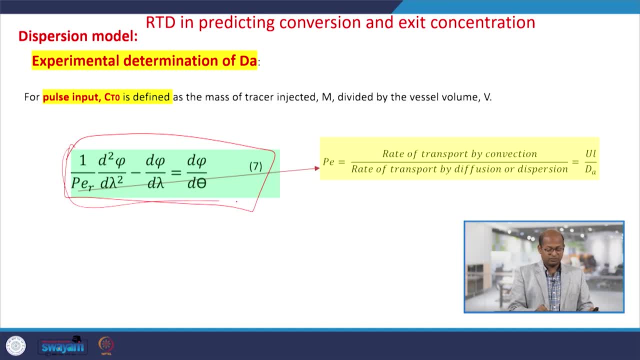 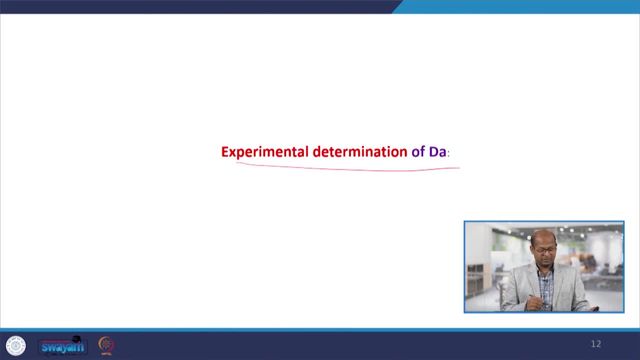 So this is time. jet and concentration is there. So therefore 3 components we have to use. So this: once we put then unsteady state, tracer, balance equation should be like this: So equation 7 is the dimensionless form for tracers. So equation 6 I think we have derived for dimension. This is dimensionless equation. 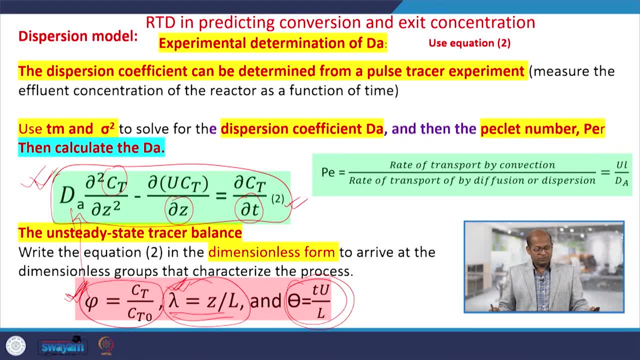 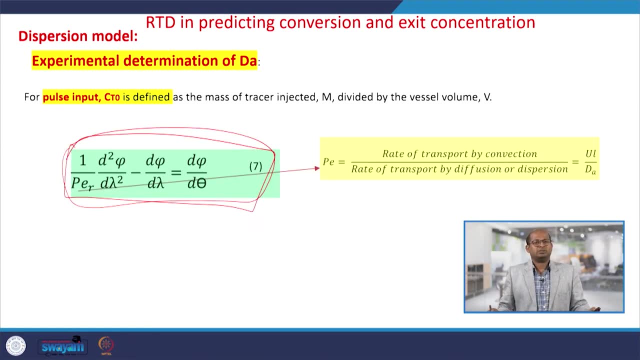 for concentrations or reaction component A. So now these two equations we can solve by using some boundary conditions. Once we have some boundary conditions to solve this type of second order differential equations, dimensionless second order differential equations- then we can solve these equations. and that we have to find out means: what are the boundary conditions? 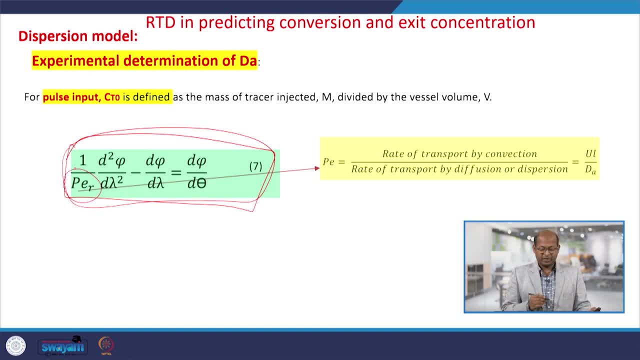 we can use to solve this equation. First we can get Peclet numbers. So then Peclet numbers means dA or diffusion coefficients. we can get if there is a diffusion or diffusivity that affect in when molecule is moving from one point to the another point. So this means non-identity. nature is there. So with the 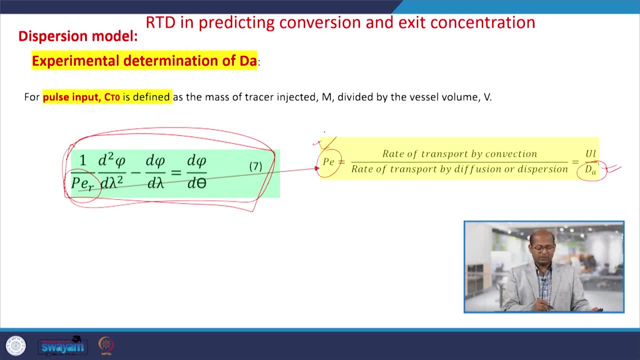 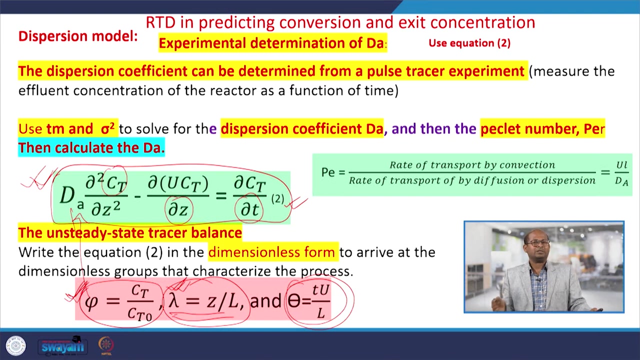 help of that means with the dA or Peclet numbers, we can say that whether dispersions affect the reactors or not, or if it is dispersion is there, Then the reactors will be able to be. So these are the two things we need means whenever we conduct any tracer test for a. 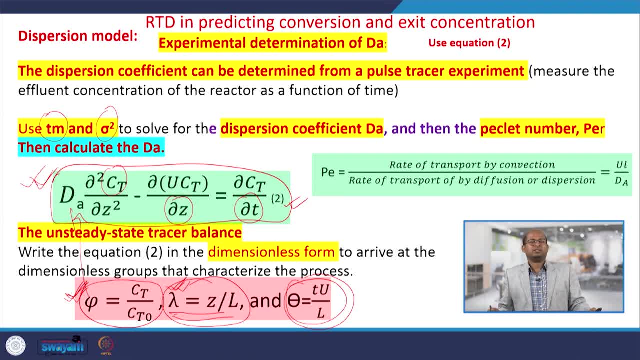 particular reactor. So tracer pulse, tracer injection should be theirs, and once tracers will come out from the reactors, So then we can measure the concentration at different time intervals, and with that we can develop C-curves, after that we can E-curves, or residence time distributions. that 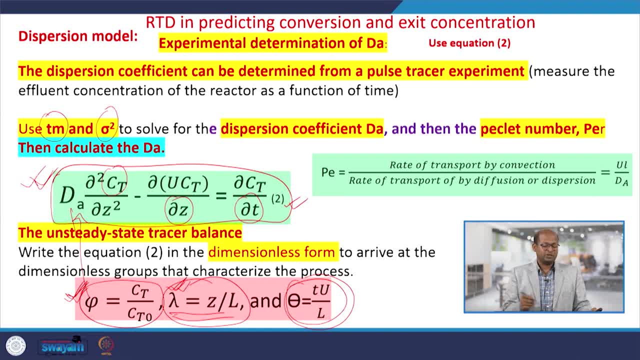 we can find for the reactors. once we know that, then mean times we can find out using that experimental data for the treasures. Similarly, sigma squares also, we can find out. that is the variance for the systems. Again, these are two known. so then, with the help of these equations, means equation 2 or 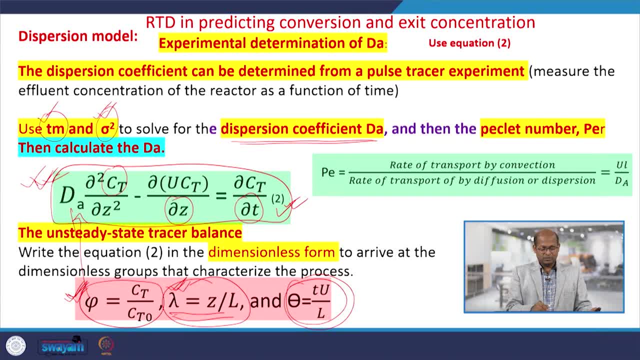 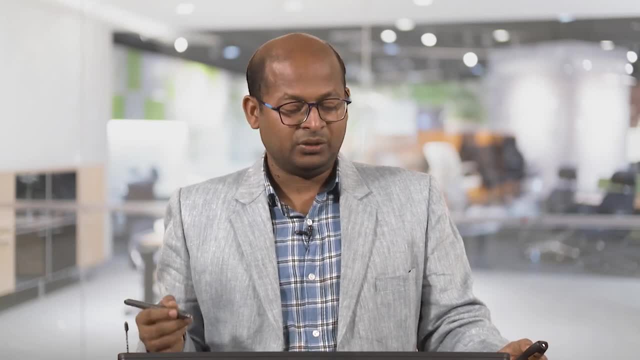 equation 6 or equation 7 also we have developed. So using this dispersion coefficient, or DA, we can find out, or Peclet number, we can find out either one. So once we know that either ones we can evaluate. So I think it is clear to you means how and what we are means differential equation, how. 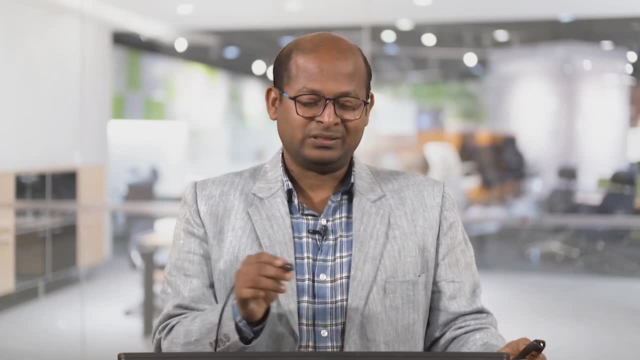 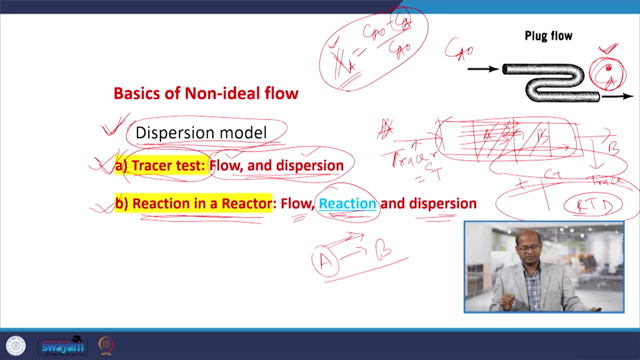 we have derived. So again Next, I am just revising or summarizing the things we have discussed. So here I said the dispersion models we are discussing. So for a reactors, when we have considered a reactors, both the way we can test the reactors, 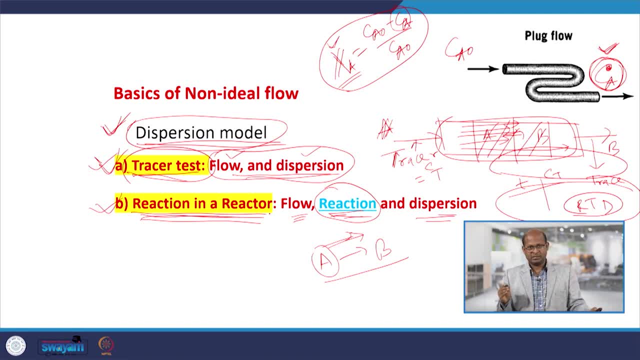 by considering treasure test and by considering flow, the reactant, reactant A, then reaction should be there if there is a dispersion. So then if treasure test is there, treasure is the non-reacting materials- there will be no reactions, only we can see flow and dispersion. 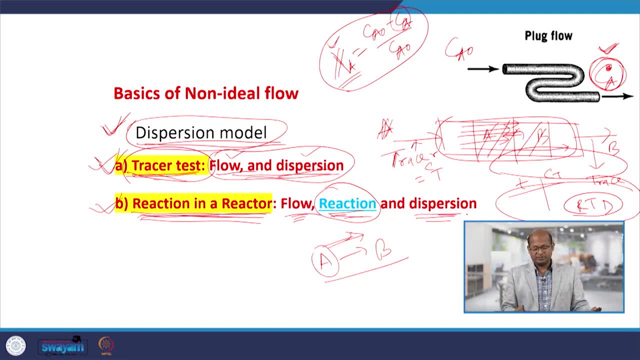 When reactions is there means reactant is passing flow, dispersion should be there. in addition to that, reactions also would be there. So how the dispersion should affect when reactions we are conducting inside of the reactors means reactant molecules diffusions might. possibility is there. So how the diffusion should affect overall performance of the reactors or the reactors. 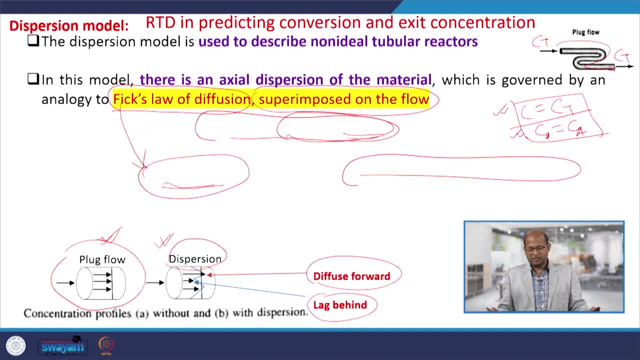 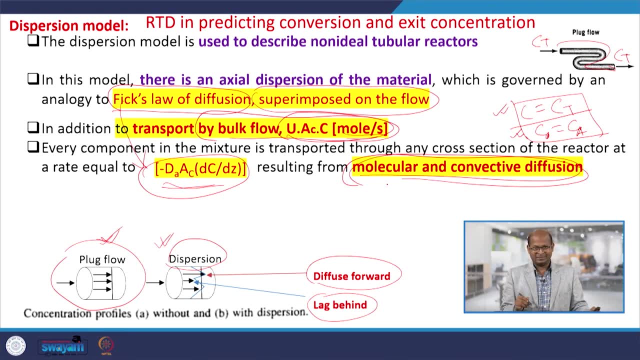 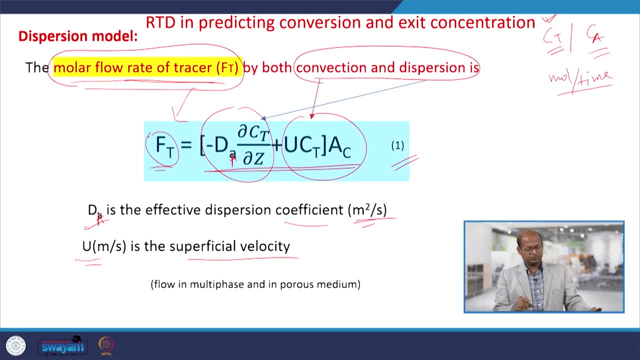 would behaves, non-ideal natures. So that things we have discussed. Thank you Next for that. we developed equations. so by considering Fick's law and molecular or convective diffusions, that things we have considered, and coupling that two So we will develop means coupling that two we can get. this is the molar flow rate when. 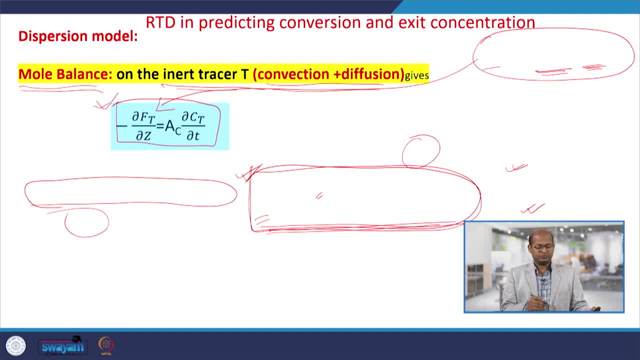 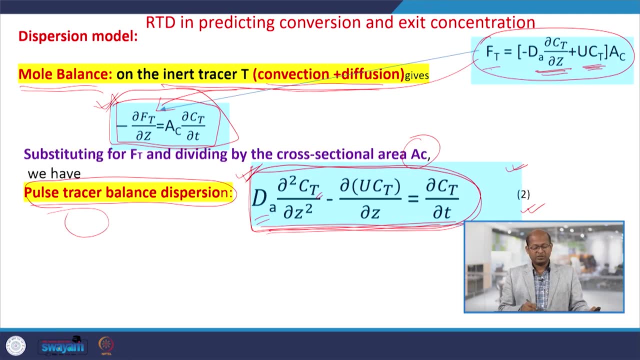 convective flow is there and diffusion is there and after that. so we have taken mole balance equation for the treasures and there is that molar flow rate, we have substituted and then we have derived the second order differential equation for treasures. Okay, So this equations we have derived and later this equations, equation two, will convert it. 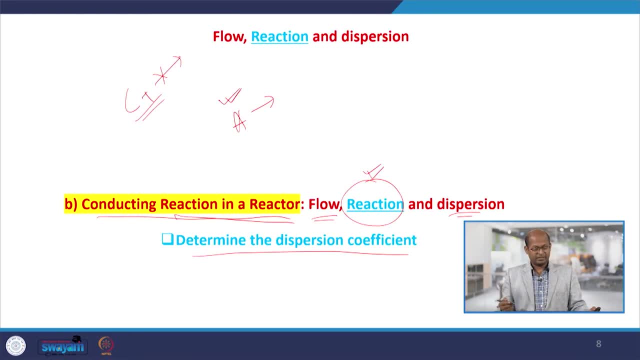 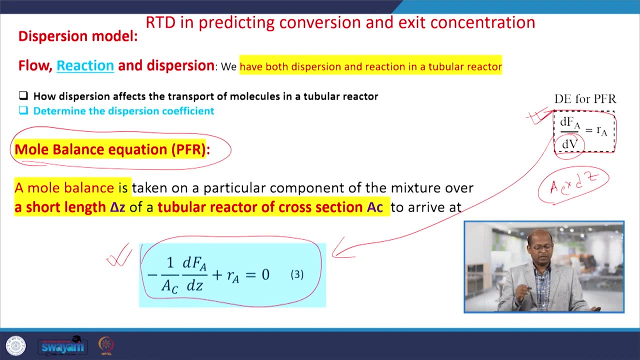 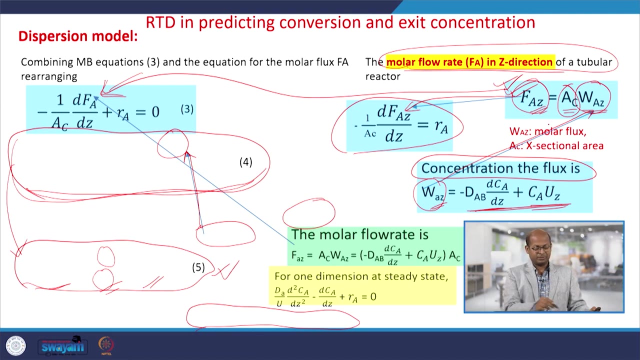 into dimensionless forms for treasures, Okay. Similarly, when reactions, is there design equations or mole balance equations? for plug for reactor we have considered, there is the molar flow rates that we have used, this molar flow rate Fz that we have substituted there, and then this second order differential equation have. 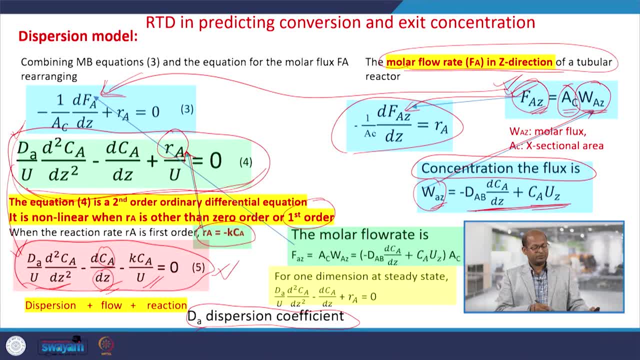 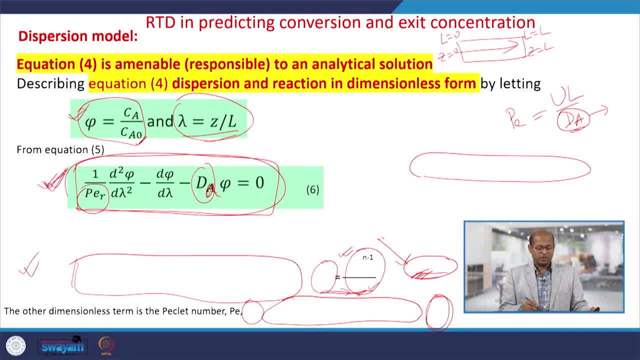 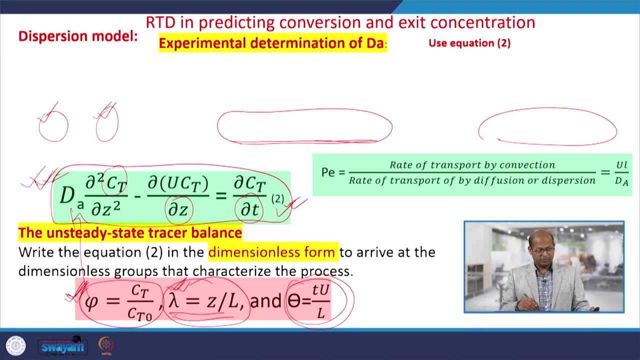 derived, Okay. Now we have simplified that equations, Okay, And by putting first order rate equations and then we have converted that into dimensionless form. So that is the equation six. So equation six is the dimensionless forms for the reactions, and another one is the this: 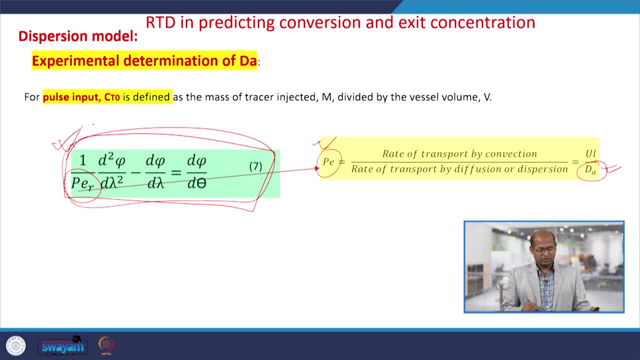 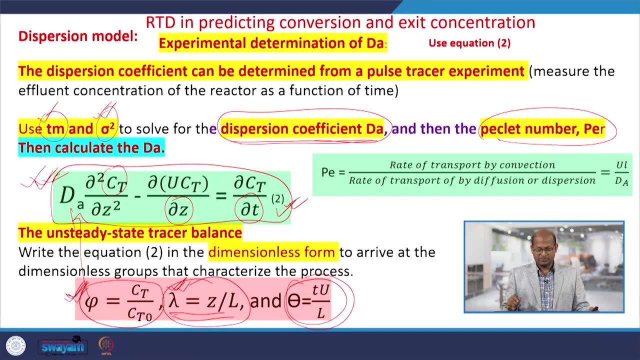 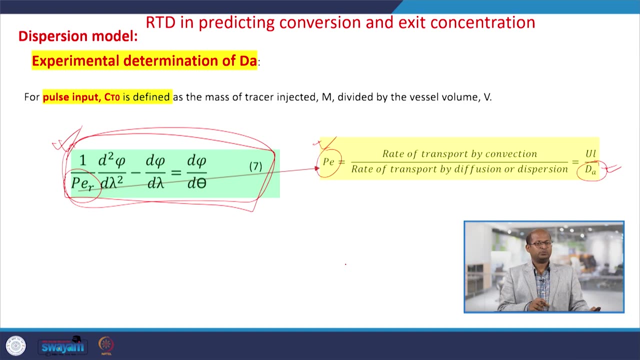 is the treasure test and for that, dimensionless, equation seven, So equation seven and equation six, So equation six and seven. both are very important. So these are the two equations. Okay, So these are the two equations that we have derived So far means how to derive the second order differential equation from treasure test and. 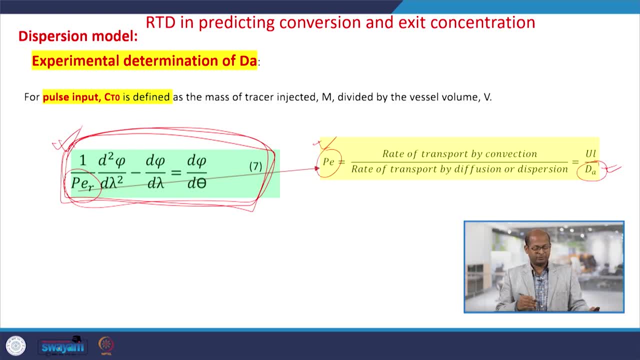 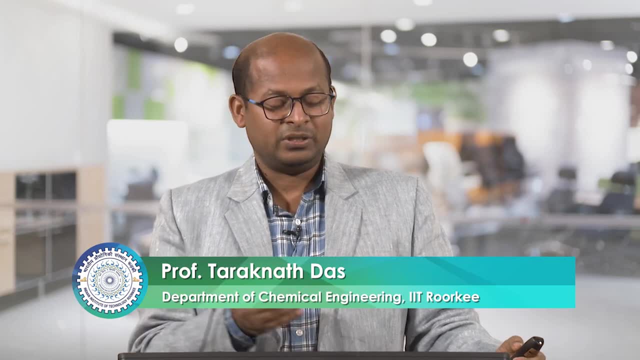 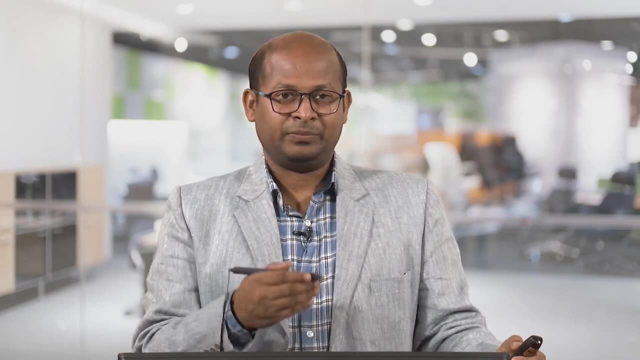 for the reactions that we know and we derived that. Okay, Now in the next class we will discuss means how these two equations we can solve, considering two boundary conditions means each equations we have to solve and for that we have to need boundary conditions So that we will discuss and then final general equation, but solutions, how that is coming.